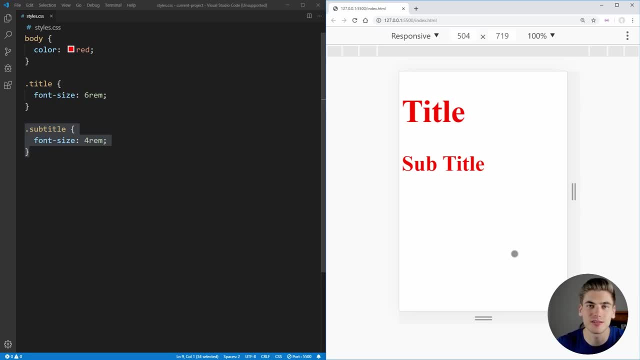 you can click on the link in the description to learn more about web design. A mobile device or a smaller screen size than a desktop device And, as I mentioned in the beginning of this video, I'm going to be talking about mobile responsiveness and you need to use media. 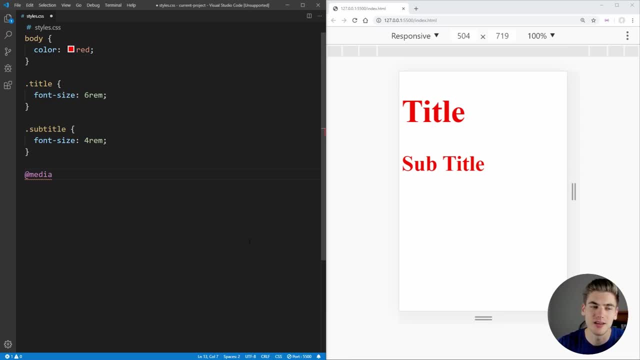 queries. in order to deal with mobile responsiveness And a media query, you just start with at media and then afterwards you need to put the type of device that you're dealing with. So this is going to be either a screen, a print device or a speech device. So screen would be. 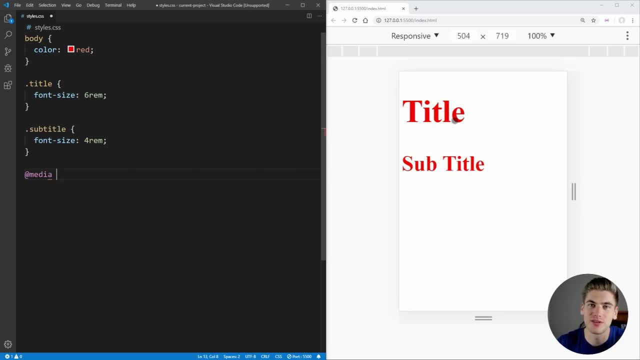 anything with a screen. For example, desktop phone doesn't have a screen, So you can use a screen, but it doesn't matter. Speech would be something that's text to speech, for example, so a screen reader, And then we have print, which would be if we tried to print the page. So if I came in here, 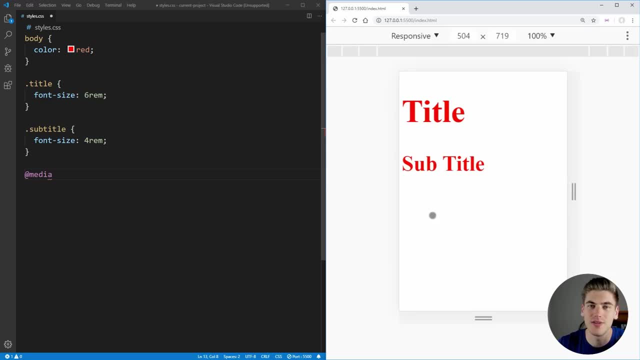 and tried to print. that would be what this section is over here. And then if you want to just select all the different types, there's also the all keyword. So most of the time you're going to be using all with your media queries- Then what you can do is you can say: and because you want to, 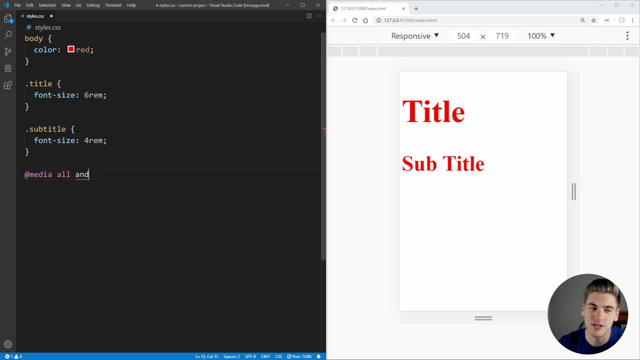 concatenate this, so you're going to say all of the screens, so any screen type, and then inside parentheses here we need to put our actual media query selector, And one of the most common types of media queries is based on width, So we can say max width of 500 pixels, for example. 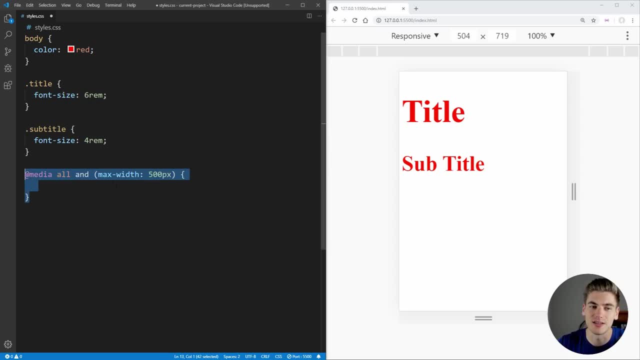 then, inside of these brackets, you just need to write normal CSS code So we can come in here and we can change the color on the body to blue. And now, if we save this, what this is saying is: whenever, on any type of screen, whether it's a screen reader, a actual screen printing- 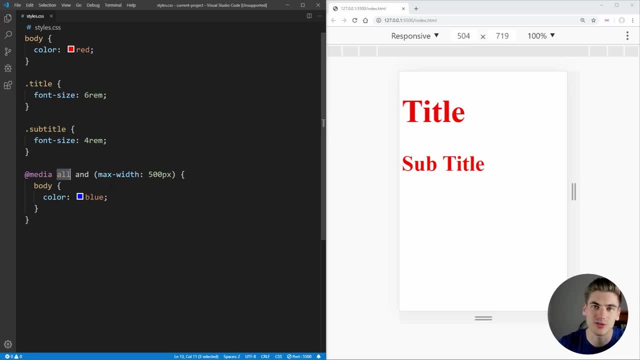 it doesn't matter, And we have a max width of 500 pixels, So essentially anything that's less than 500 pixels wide and, as you can see, we're at 504 pixels. So when we shrink this, you can see our text turns blue below 500. And it turns back to red above 500. And that's because 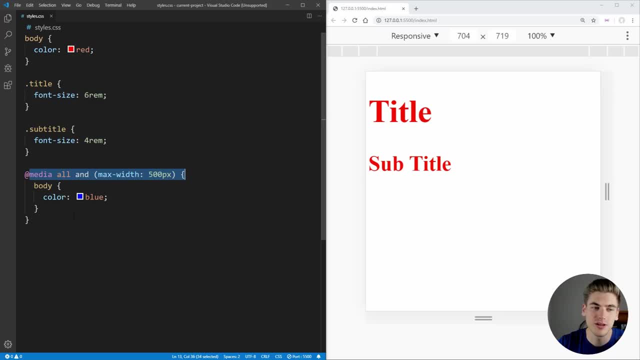 what this media query is doing is. whenever all of these values are true, then the code inside of it is actually run. If any of the values are false, it just ignores everything inside the media query. And now one thing that you'll notice is: a lot of times you 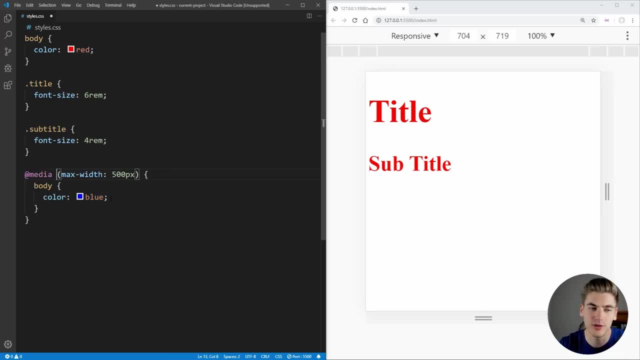 don't see this all keyword, And that's because you're not going to be able to see this all key word. And that's because if you remove the all at the beginning, it defaults to all. So if you want to do a media query on all different types of devices, you can just leave out the all and just. 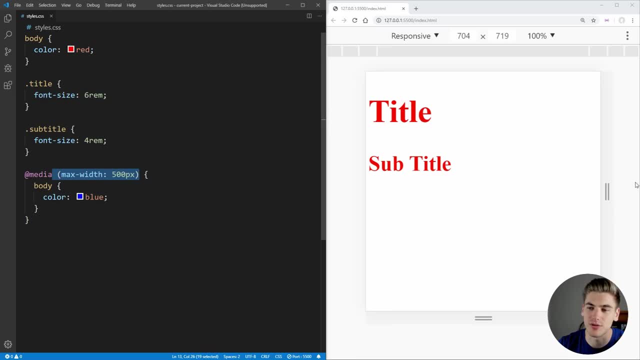 put in the parentheses section, for example, max width of 500 pixels And, as you can see, that works just as before changing our text color. for us. Another thing that we can do is print specific styles, So we can say a media query for print. 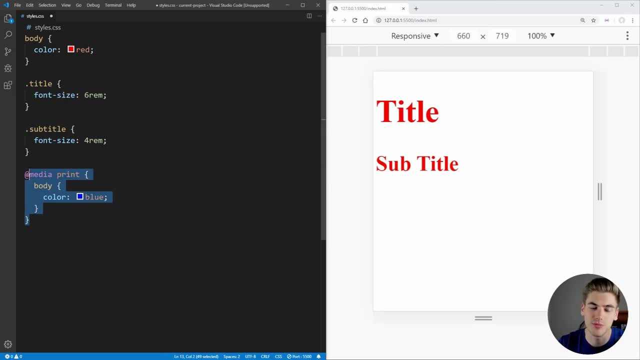 we can just remove this parentheses section because we just want- anytime we're printing, we want the color to be blue. Now, if we save that and we go to print, you'll see that our text color is blue for printing, which is great. One thing to note about media queries is that they work just like other 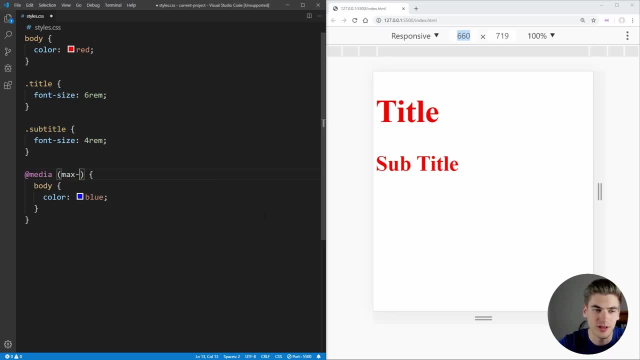 selectors. So if we change this here back to a max width of 500 pixels, save that and make sure that still works. Yep, still blue below 500.. And right above: if we change this body selector and we move it all the way down below our media query, you'll notice that, no matter what screen. 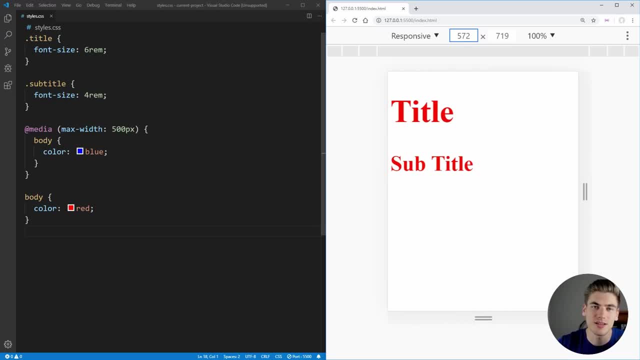 size we're on. If we move it all the way down below our media query, you'll notice that, no matter what screen size we're on, it just always going to be red text. And that's because it's reading from top to bottom, And it's always. 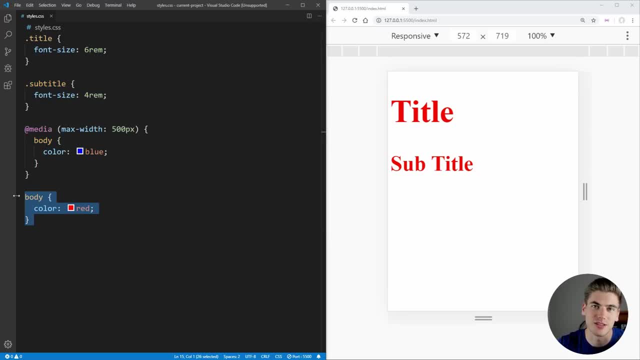 going with the bottom selector if the selectors have the same specificity. So it's going with a red color, even though this blue color is in the media query. Essentially it just ignores it because there's another selector after it. Now let's move that body selector all the way back. 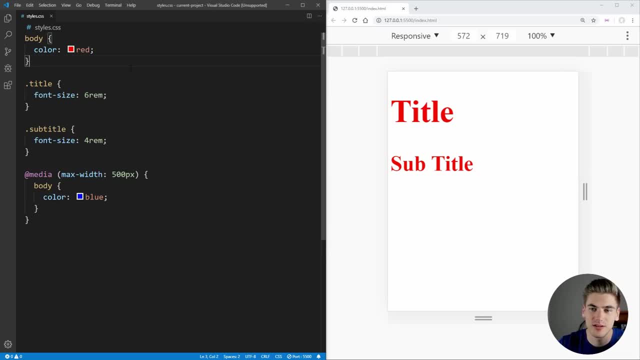 to the top So we can have actual working code And if we save that, you can see that it's now working again. we have our blue text and our red text. Another thing that we can do is inside of our media we can actually change the color of our text. So if we go to print we can see that it's 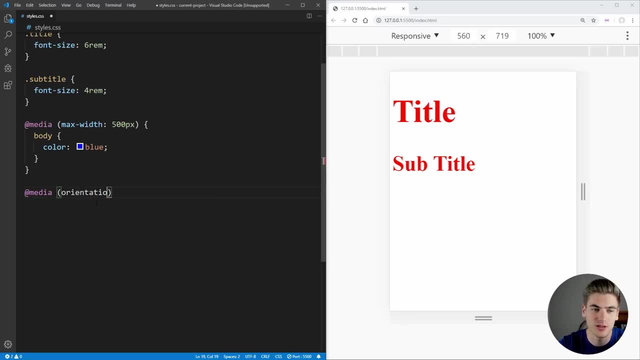 actually dealing with the orientation of our device. So we can say orientation And we want to do, for example, landscape. So whenever we're in landscape mode- essentially horizontal mode, what we want to do is we want to change our title to have, for example, a color of will go with. 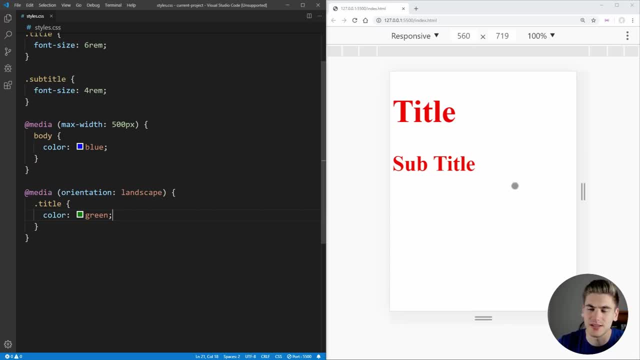 green. So now, as you can see, we're not in landscape mode, we're in portrait mode And our text is normal. And as soon as we go into landscape mode, essentially whenever our width becomes wider than our height, as you can see here, our text color has changed to green to match that orientation of landscape. 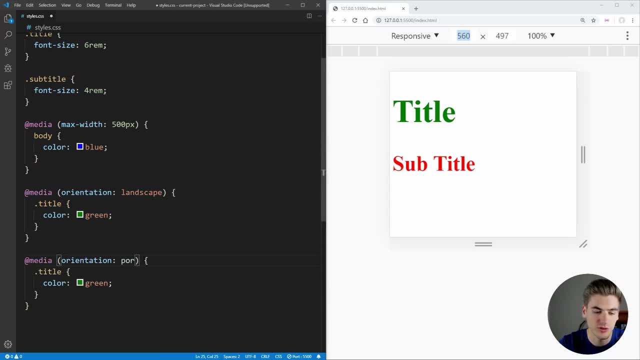 we can also do a very similar thing, But we can do portrait instead, And in this one we'll just change our subtitle to be cyan. And now, as you can see, when we go into portrait mode our subtitle changes to cyan, And in orientation mode, you can see, our title is green. we can even go as far as 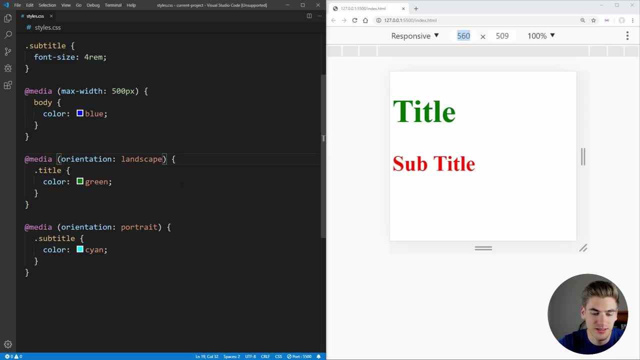 to combine these together. So, for example, we can say when we're in landscape mode and when our max width is going to be 500 pixels. So now, as you can see, we are in landscape mode, but our width is above 500 pixels. As soon as we drop it below that, you can see that we've changed to that green text. 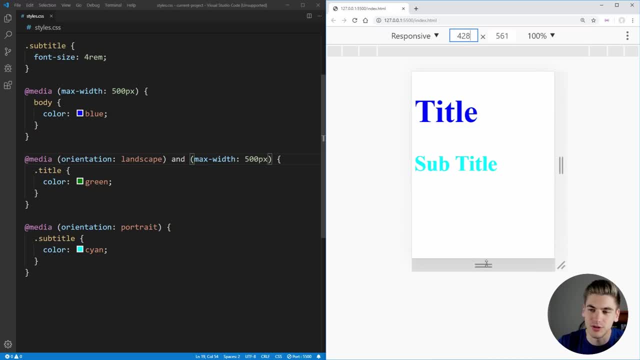 And then, once we leave landscape mode, you can see it goes back to blue. So we had to both be in landscape mode and be less than 500 pixels wide, because we're able to concatenate these with the and keyword. If you wanted to do an or statement instead of, and we could do is just put a comma. 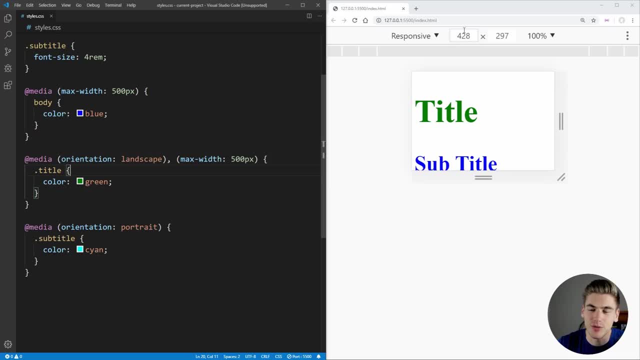 instead of the keyword: and. And. that's going to change our text color to blue, And then we can see that we're in landscape mode. So now, what this is saying is, anytime we're under 500 pixels or in landscape mode, it's going to be green. So, as you can see, we are not in landscape mode. 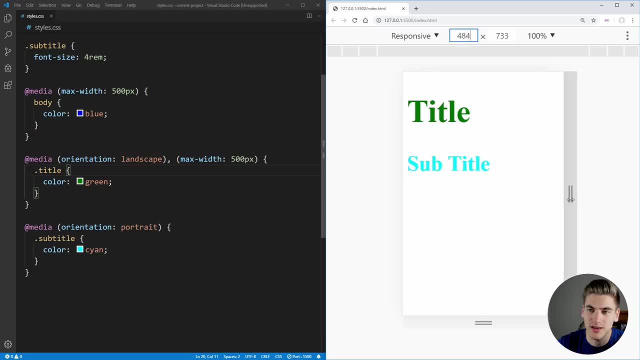 anymore, but our width is less than 500 pixels, So it's green, And as we increase that above 500.. Now we're no longer in landscape mode and no longer less than 500 pixels wide, So it's going to be red. But as soon as we enter landscape mode, even though we're not less than 500 pixels, it's. 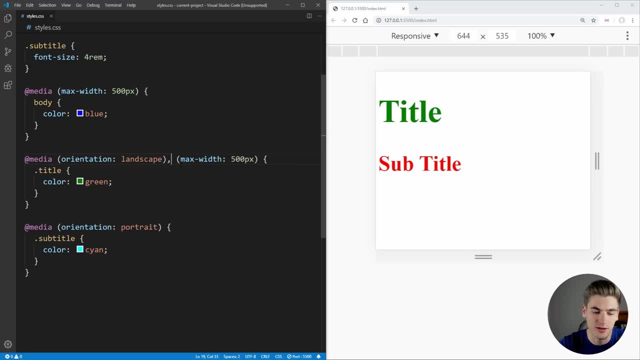 going to turn into green. So you remember, comma is going to be for an or an and is going to be for, and There are quite a few different selectors that you can use with media queries, But really the main ones that you're going to mess with is going to be orientation, print and max or min width, And 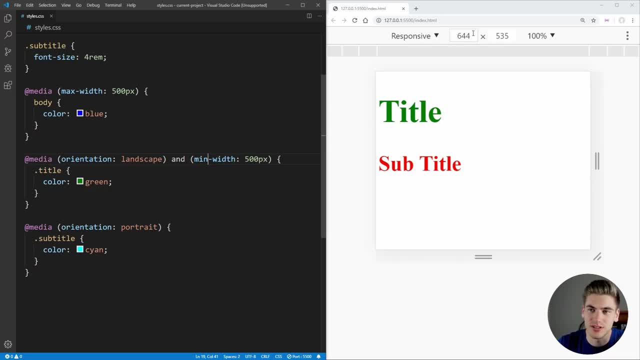 min width is obviously just going to be the opposite of max width. So, as you can see, we're over 500 pixels wide and we're in landscape mode, So it's going to be a title of green, And as soon as we leave that landscape mode or we become less than 500 pixels wide, it's obviously no longer. 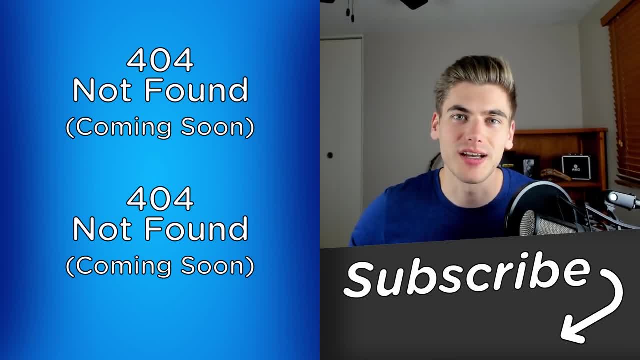 going to work, And that's all there is to responsive design with media queries. If you enjoyed this video, make sure to check out my other videos which are going to be linked over here, And also subscribe to the channel for more videos just like this one. Thank you very much for.